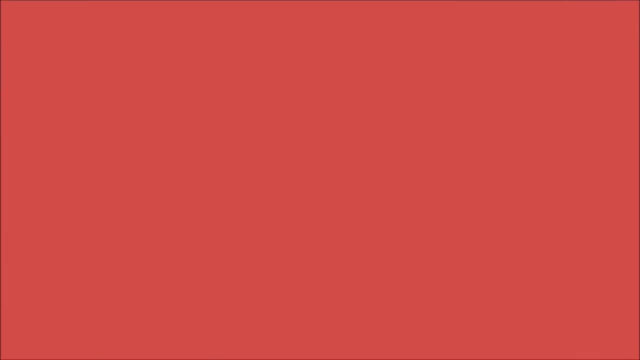 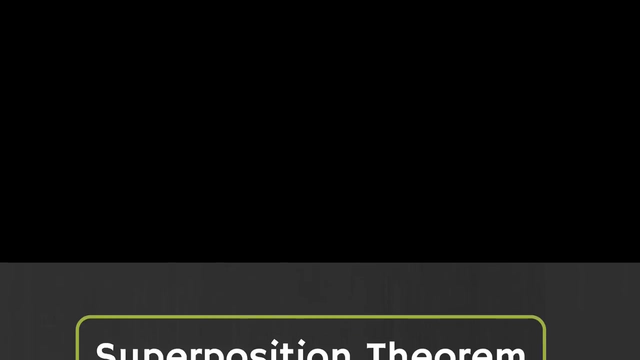 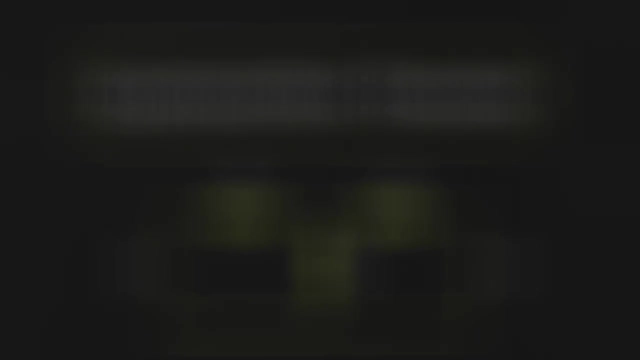 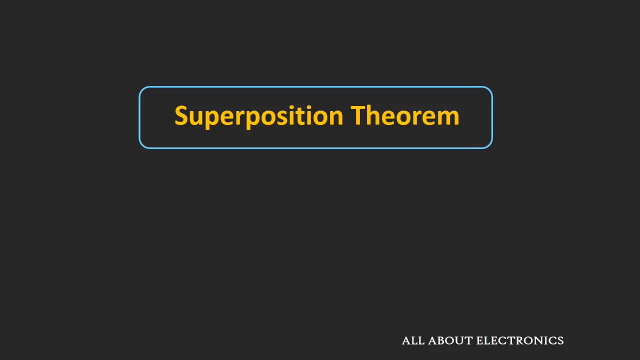 Hey friends, welcome to the YouTube channel ALL ABOUT ELECTRONICS. So in this video we will learn about the superposition theorem in the electrical circuits. So in this video we will see some features of this superposition theorem, like under which condition this superposition theorem can be applied, what is the usefulness of this superposition. 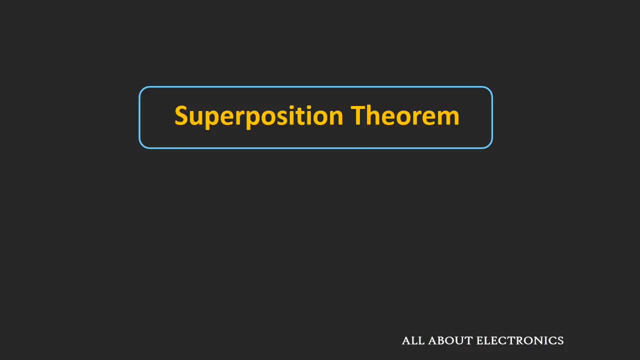 theorem, what are the limitations of this superposition theorem, and we will solve some problems based on this superposition theorem. So we will understand this superposition theorem by taking one example. So, as you can see, here we have total two. 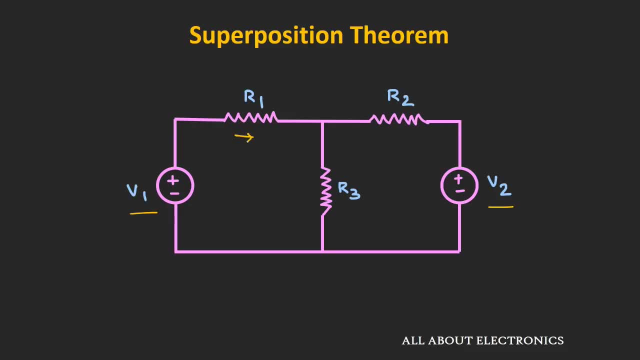 independent voltage sources And let's say we want to find the current I that is flowing through this resistor R1. So, using this superposition theorem, what we can do, we can consider this one particular voltage source or one particular independent voltage source at a time, And we can find. 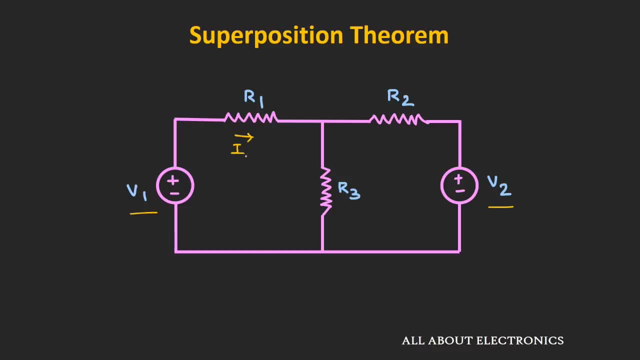 the current that is flowing through this resistor R1.. So suppose, if we consider this voltage source V1 alone, then we can turn off this voltage source V2.. And we can replace this voltage source V2 by their internal impedance. Now here all the independent voltage sources that we are considering are ideal sources. 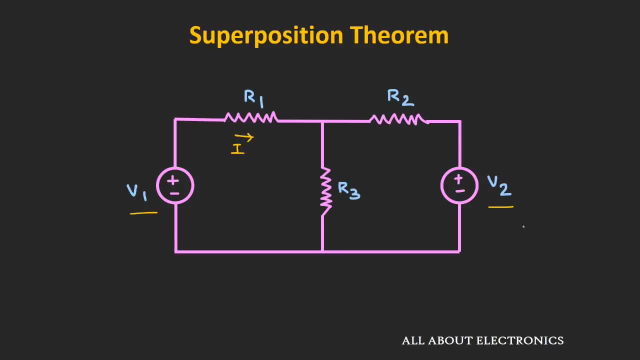 So the ideal voltage source has a zero series internal impedance. So we can replace this voltage source V2 by a short circuit. So in this case we can find the current that is flowing through this resistor R1. Let's say the current that is flowing to this. 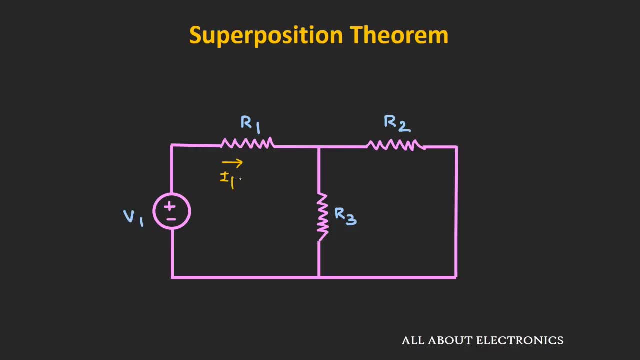 resistor R1 is I1.. Similarly, in the second case, what we can do: we can consider this voltage source V2 alone and we can turn off this voltage source V1.. So we can replace this voltage source V1 by a short circuit. 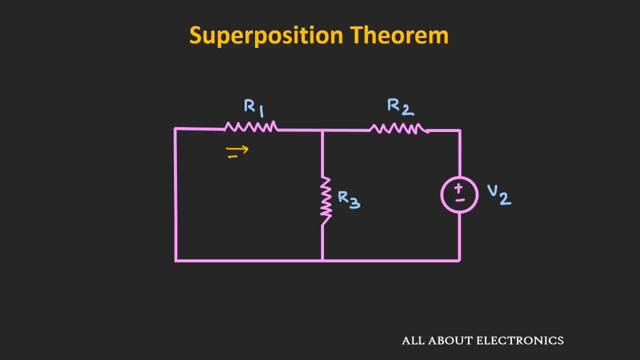 And in this scenario we can again find the current that is flowing through this resistor R1.. Let's say, in this case, the current that is flowing through this resistor R1 is I2.. Now, the total current that is flowing through this resistor R1 will be nothing but the algebraic. 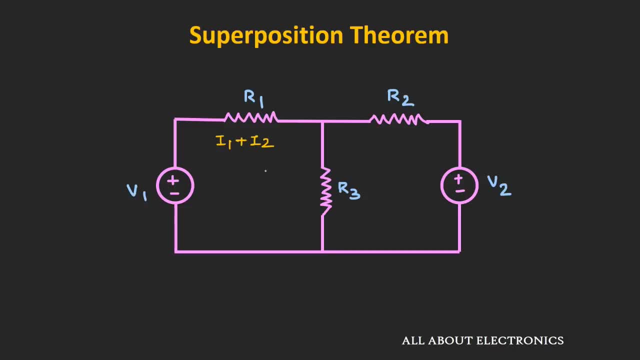 sum of this current I1 and I2.. So the total current that is flowing through this resistor R1 is nothing but the algebraic sum of this current I1 and I2.. So, according to the superposition theorem, in any linear bilater network containing more 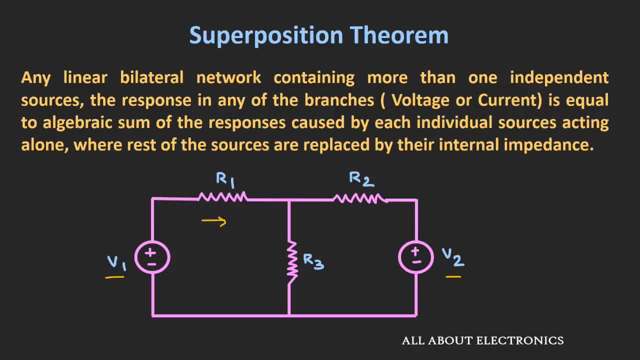 than one independent source. the response in any particular branch- either voltage or current- that is equal to the algebraic sum of the responses that is caused by individual sources acting alone And at the same time all the other sources are replaced by the internal impedance. 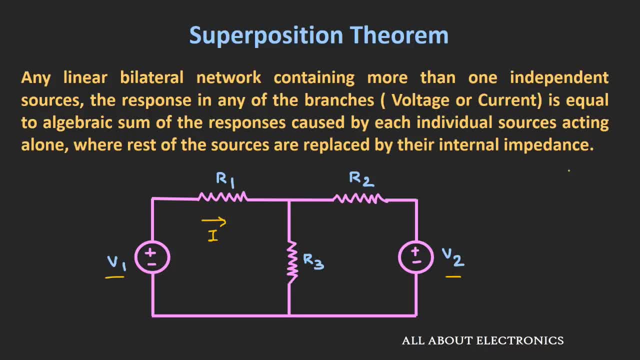 Now, in most of the cases, as we are considering the ideal sources, so all the ideal voltage sources can be replaced, All the ideal current sources can be replaced by the short circuit, and all the ideal current sources can be replaced by the open circuit. 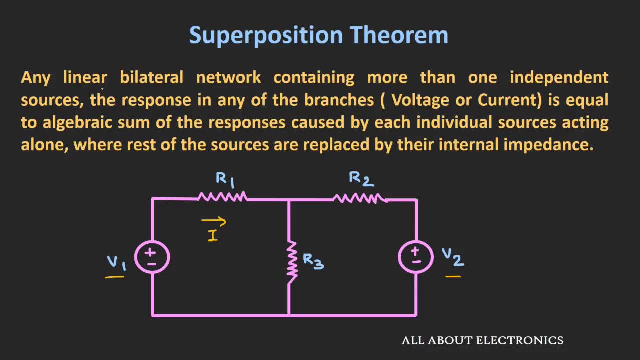 So now, in this statement, if you see, we are considering a linear bilater network, So this superposition theorem can be applied only for the linear and the bilater network. Now, if you don't know about this linear and bilater network, then you can check my video. 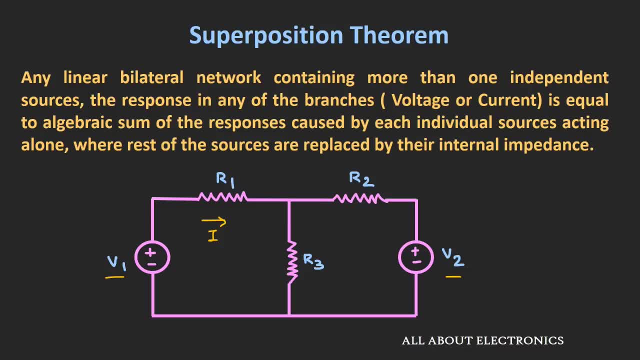 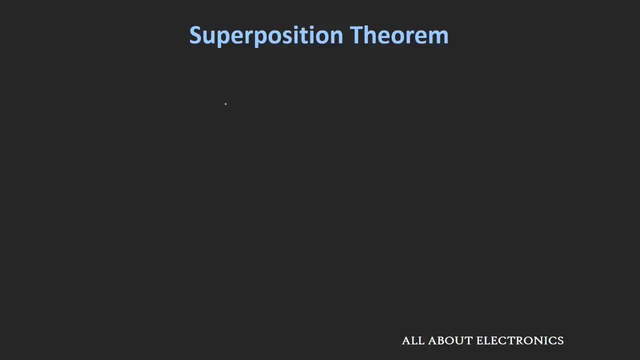 on the classification of the electrical network. The link for the same I will provide in the description below, So you may check that out. So now let's see some features of this superposition theorem. So, as I said earlier, this superposition theorem is only applicable for the linear and the 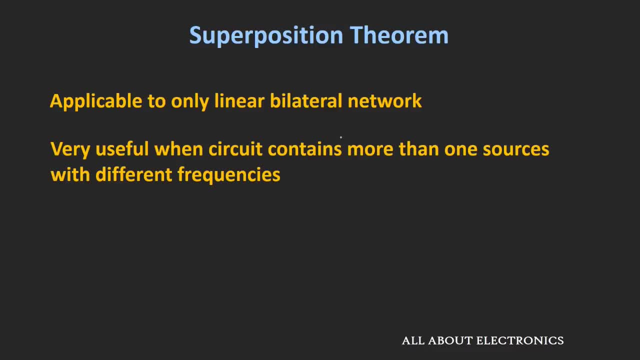 bilater networks. Now this particular superposition theorem is useful when the circuit contains more than one source with different frequencies. Now if your circuit contains only DC sources, then there are many ways you can find that solution. But if the circuit contains AC sources, and also with different frequencies, then this: 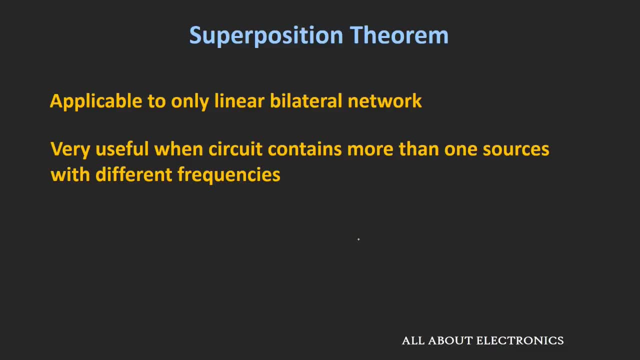 superposition theorem is quite useful. So let's see some features of this superposition theorem Now, apart from the independent sources, if the circuit contains dependent sources as well, then those dependent sources will be considered on during the analysis. So this will get clear to you when we'll take one example based on this dependent source. 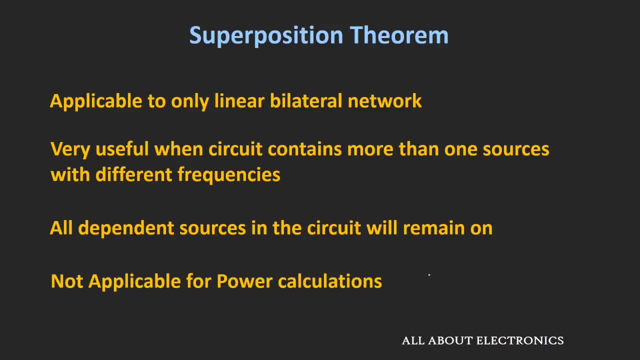 So now, this superposition theorem is not applicable for the power calculations, So we will understand more about it when we'll take one example based on this power calculation. So now let's see some examples based on the superposition theorem. 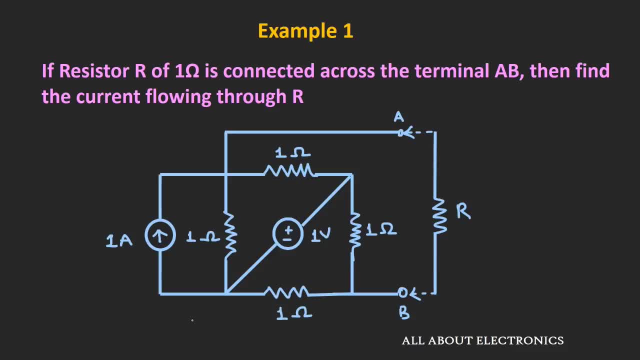 Now in the first example. So in the first example, given this electrical circuit and we have been asked to find the current that is flowing through this 1 Ohm resistor, So we will solve this example using this superposition theorem. So what we will do, we will consider only. 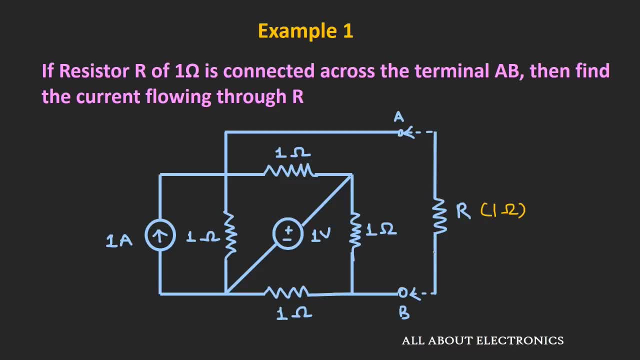 one particular independent source at a time And because of that independent sources, we will find the current that is flowing through this resistor R And the algebraic summation of those current will be the total current that is flowing through this resistor R. So first of all, let's consider this: 1 Ampere. 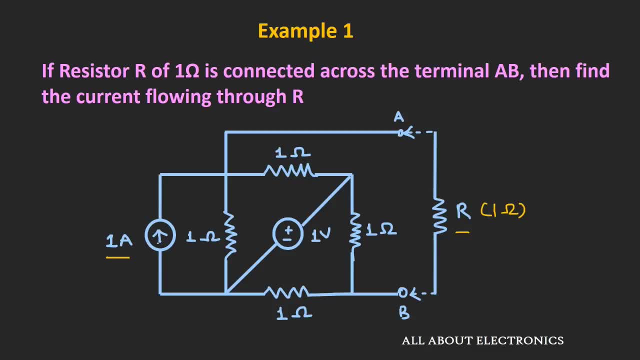 current source. So now suppose, if we consider only this 1 Ampere current source, only then this voltage source will get short circuited. And if you see the equivalent circuit, the equivalent circuit will look like this: So now in the equivalent circuit, if you see, these two 1 Ohm resistors are in a parallel. 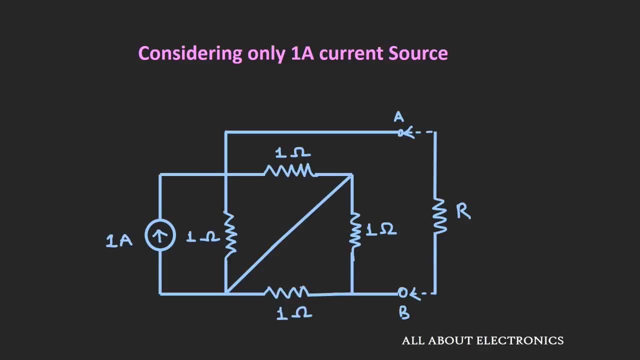 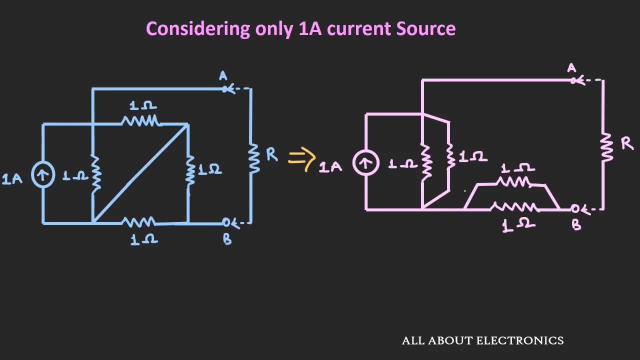 Similarly, these two 1 Ohm resistors are also in a parallel, So we can redraw this circuit like this. So now here, as these two 1 Ohm resistors are in parallel, so we can replace them by the equivalent parallel. 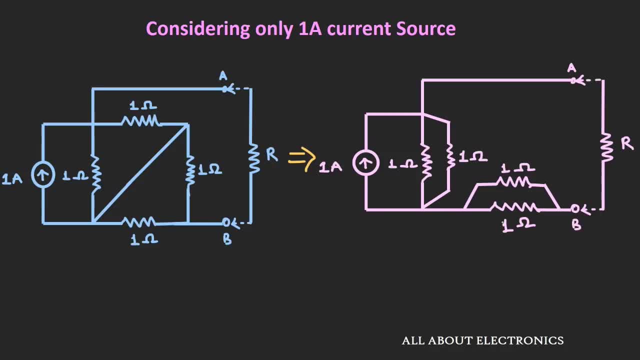 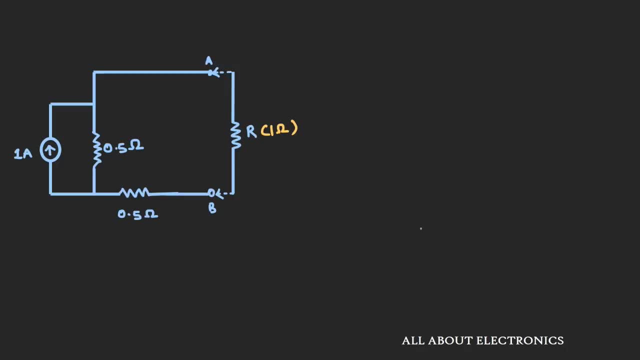 That will be the 0.5 Ohm. Similarly, the equivalent parallel resistance of these two 1 Ohm resistors will be 0.5 Ohm. So now the equivalent circuit will look like this: So now this 1 Ampere current will get divided. 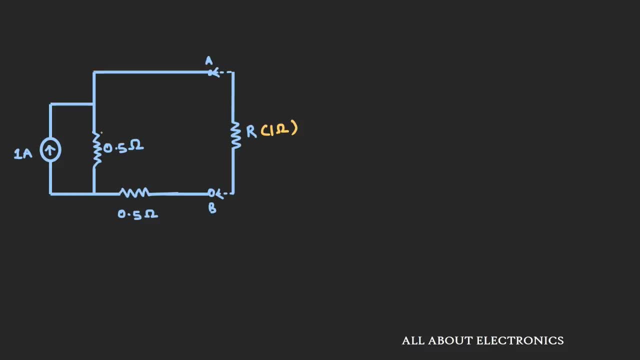 in two branches. Some portion of this current will flow through this 0.5 Ohm resistor and the remaining current will flow through this series combination of this 0.5 Ohm and a 1 Ohm resistor. So the equivalent circuit will look like: 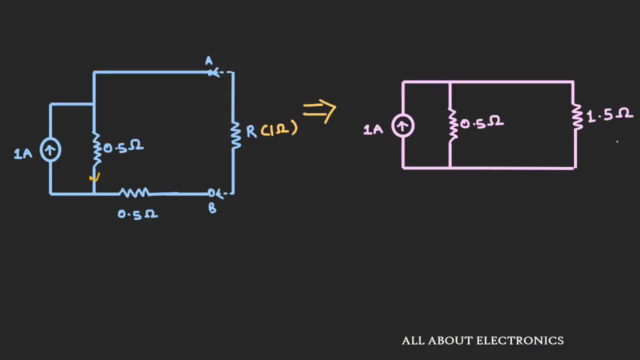 this. So the current that is flowing through this 1.5 Ohm resistor is nothing but a 0.5 divided by 0.5 plus 1.5 into 1 Ohm, which will come out as a 0.25 Ampere. This is nothing but a current divider rule. 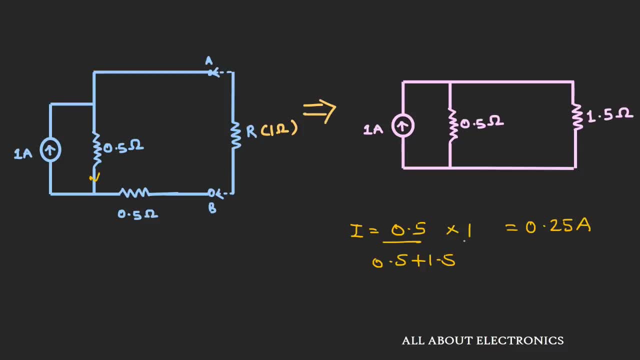 So, using this current divider rule, the current that is flowing through this series combination of 1 Ohm and 0.5 Ohm resistor is nothing but a 0.25 Ampere. So we can say that the current I1 that is flowing through this resistor R is nothing but a 0.25 Ampere. 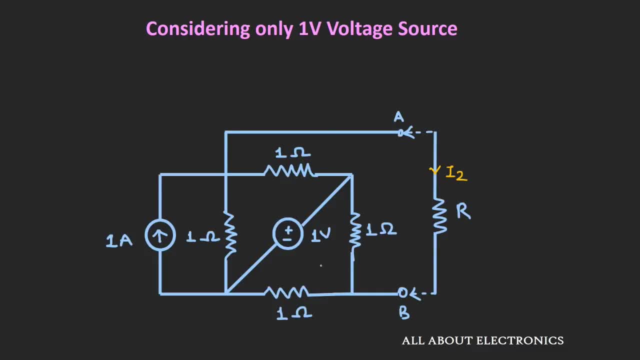 So now let's consider only this 1V voltage source And let's assume that the current that is flowing through this resistor R is nothing but I2.. So when we consider only this particular voltage source, then this current source can be replaced by the open. 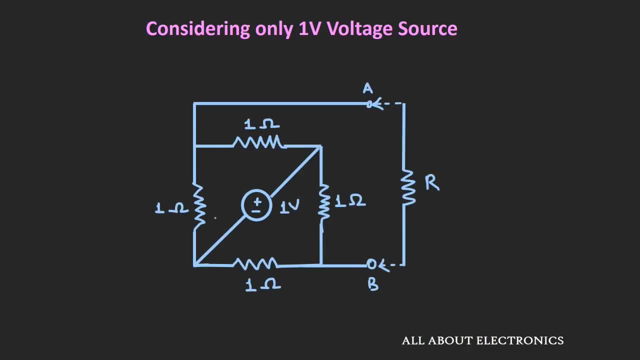 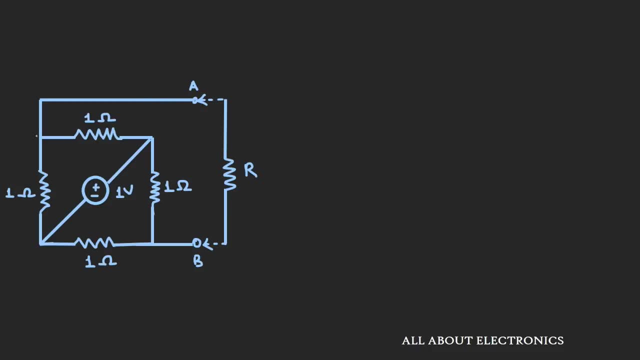 circuit and the equivalent circuit will look like this. So now let's redraw this circuit. See here, this is the terminal A. So we can say that this is also terminal A and this is terminal B. So first of all, as you can see, the two 1 Ohm. 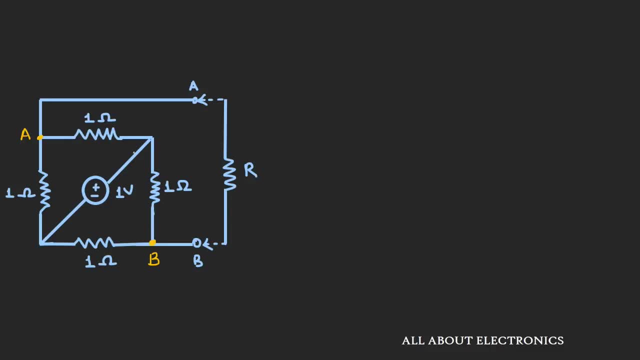 resistors are connected to this positive terminal of this 1V voltage source, So we can redraw this circuit like this. So these are the two 1 Ohm resistors which are connected to the positive terminal of this 1V voltage source, And this terminal will be nothing but an A. 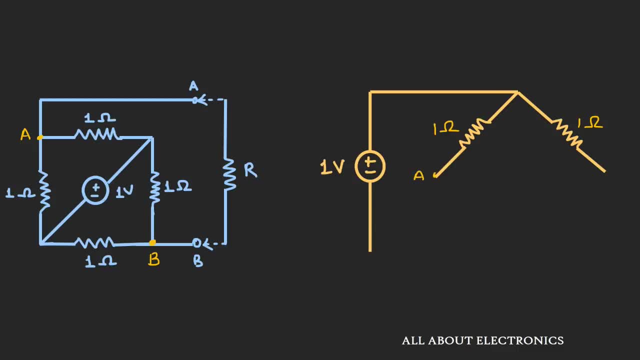 terminal, Similarly at the negative terminal of the positive terminal of this 1V voltage source. once again, these two 1 Ohm resistors are connected, So we can redraw these two 1 Ohm resistors like this. So again here this point will. 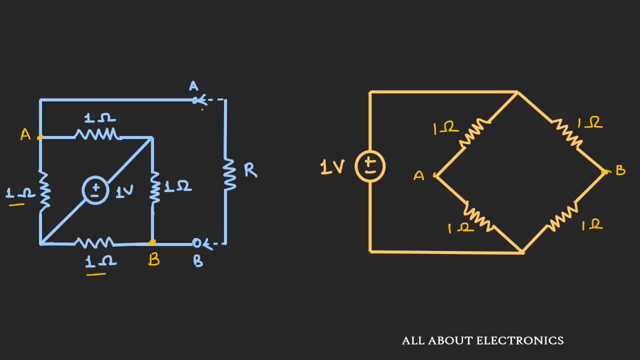 be nothing but a terminal B, And across this terminal A and B 1 Ohm resistor R is connected. So the equivalent circuit. now we can redraw like this. So now, if you see this circuit, this circuit is nothing but a balanced Whiston bridge circuit. So as this Whiston bridge 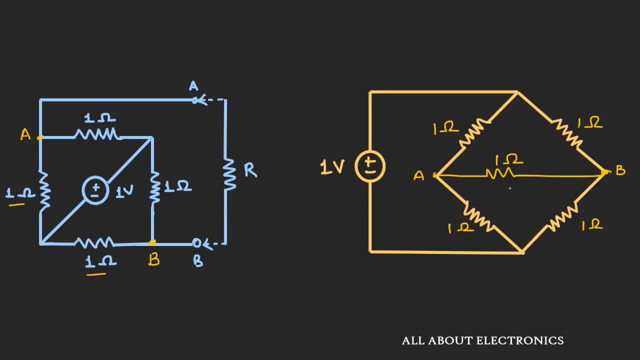 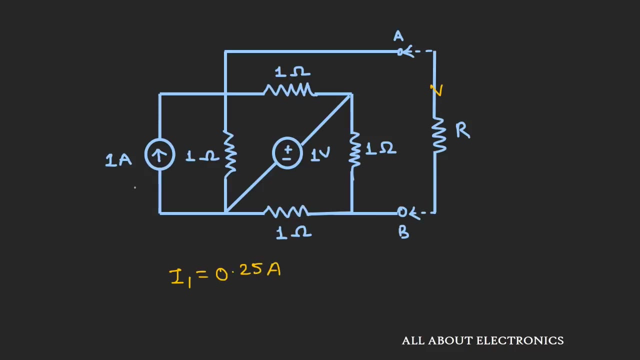 is a balanced bridge, so the current that will flow through this 1 Ohm resistor will be nothing but a zero. So we can say that the value of this I2 is nothing but a zero ampere. So in this way we found out that the current I1 is 0.25A. when this 1A current 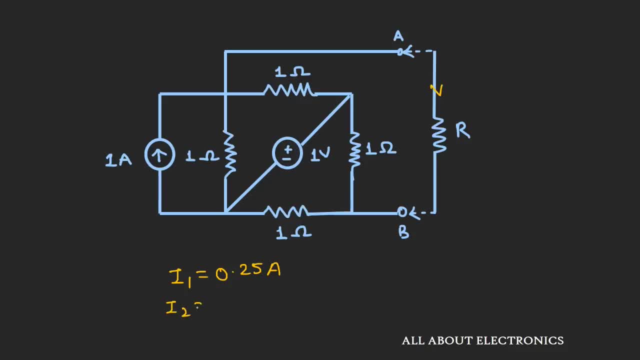 source is acting alone And current I2 is zero when this only 1V voltage source is acting alone. So the total current I that is flowing through this resistor R is nothing but I1 plus I2.. That will be nothing but a 0.25A. So in this way, using this superposition, 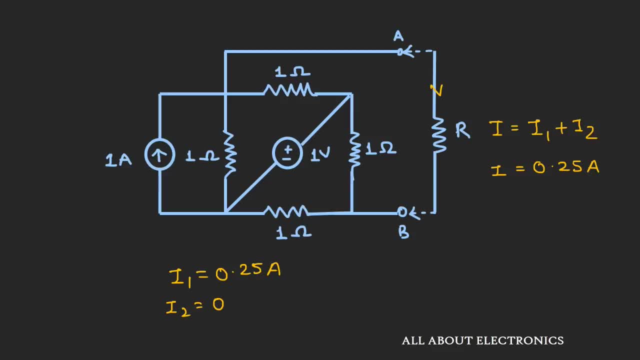 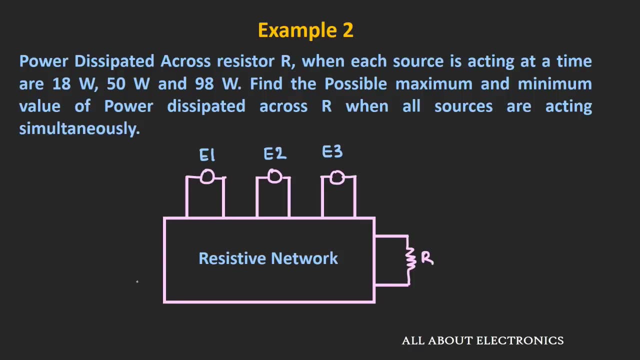 theorem we can find the total current that is flowing through this resistor R. Now let's see the second example. So in this example we have given one resistive network And in this resistive network three independent voltage sources are connected. 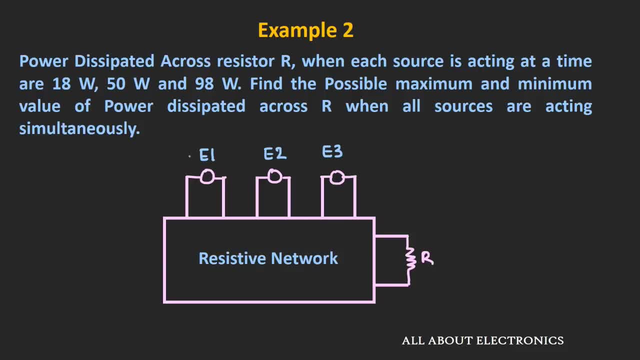 And we have given that when these independent voltage sources are acting alone, then the power that is dissipated across this resistor will be 0.25A. So we have given that when these independent voltage sources are acting alone, then the power that is dissipated across 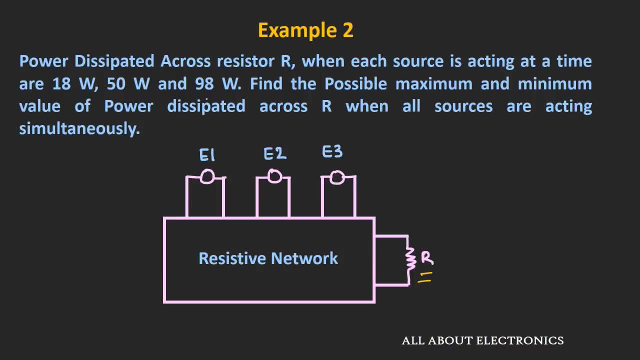 this resistor R is 18W, 50W and 98W. So we have been asked to find the possible maximum and minimum value of power that is dissipated across this resistor R when all the three sources are acting simultaneously. So here we have given that when voltage source 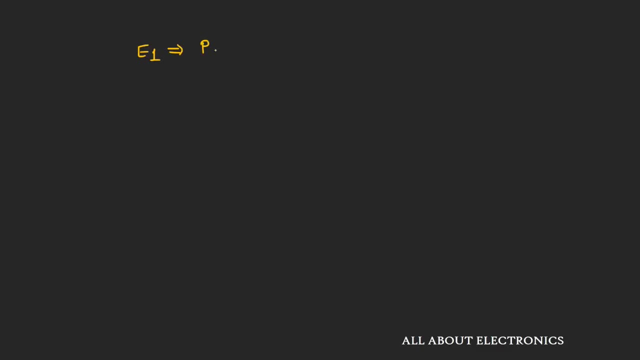 I1 is acting alone, then the power P1 is 18W. Similarly, when the voltage source I2 is acting alone, then the power that is dissipated across the resistor R is 50W. And similarly, when this voltage source E3 is acting alone, then power P3 that is dissipated. 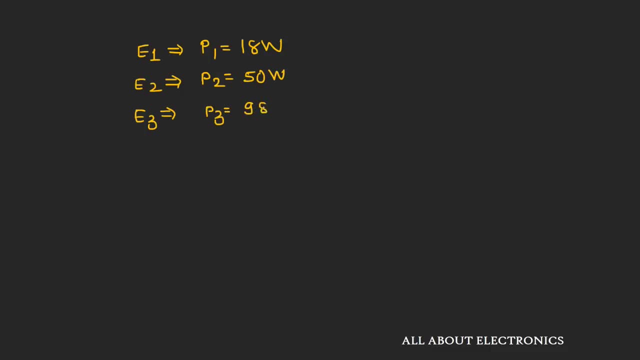 across. this resistor R is 98W. Now we can write this P1 as I1² into R. Let us say I1 is the current that is flowing through this resistor R when this E1 is acting alone. Similarly, we can write this power P2 as I2² into R And we can write this power P3 as: 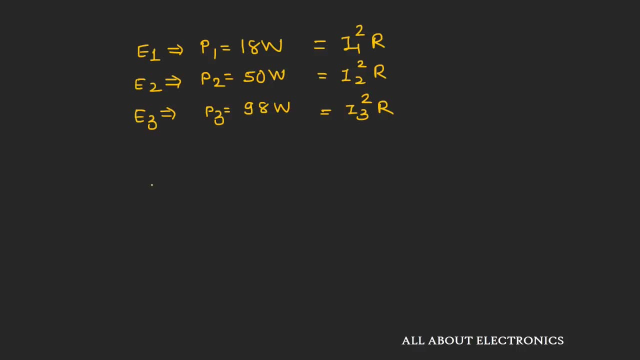 Now. earlier we have discussed that for the power calculations we cannot apply this superposition theorem. So if three voltage sources are acting simultaneously, then the total power, P1 plus P2 plus P3, will not be equal to I1 square into R plus I2 square into R plus I3 square into R. 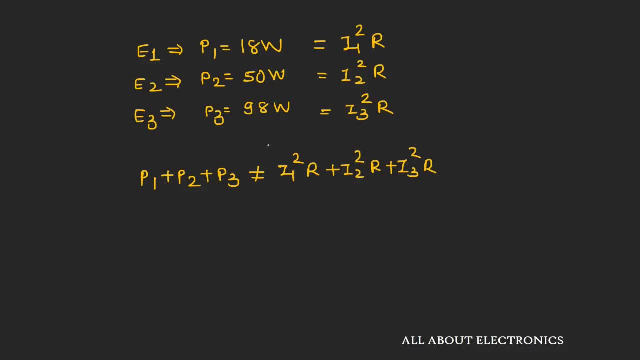 So directly we cannot add these three powers to find the total power that is dissipated across this resistor R, But rather, when the three voltage sources are acting alone, then the total current that is flowing through this resistor R, that is, I total, will be nothing. 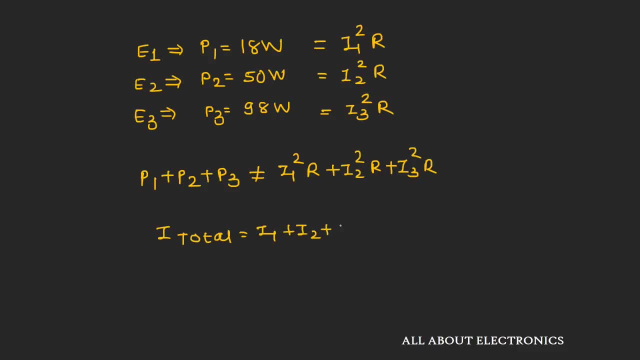 but I1 plus I2 plus I3.. So the total power P that is dissipated across this resistor R is nothing but I1 square into R plus I total whole square into R. So this will be the total power that is dissipated across this resistor R. Now here in this example, we have been asked: 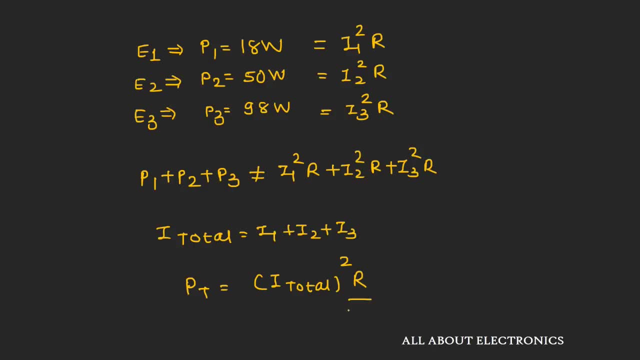 to find the possible maximum and the minimum value of this power. So, first of all, let's find the value of this: I1,, I2, and I3.. So, as we know, P1 is equal to, 18 is equal to. I square into R, So we can say that I. 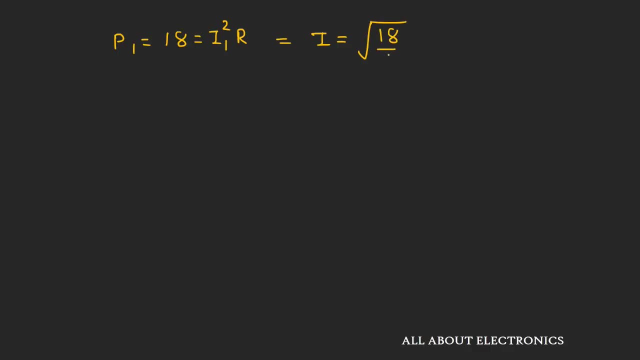 is nothing but under root 18.. So P1 is equal to 18.. Therefore we are big- sondern 18: 2 power by 2 whole square R. Similarly, I2 will be nothing but under root, 50 over R And I3 will be nothing but the under root. 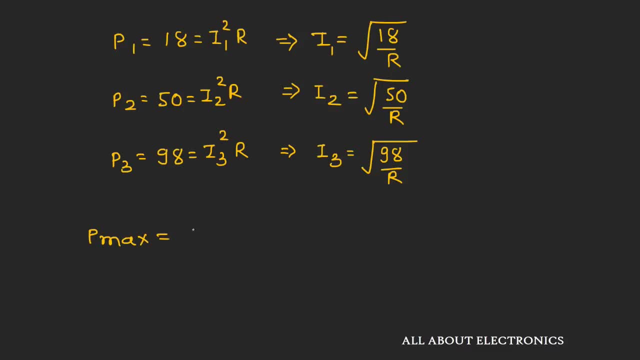 98 over R. So for maximum possible power Pmax will be nothing but I1 plus I2 plus I3, whole lab, 2 square into R, That's nothing but R18 plus plus root, 98 whole square. And if we further simplify it then we will get 2 into under. 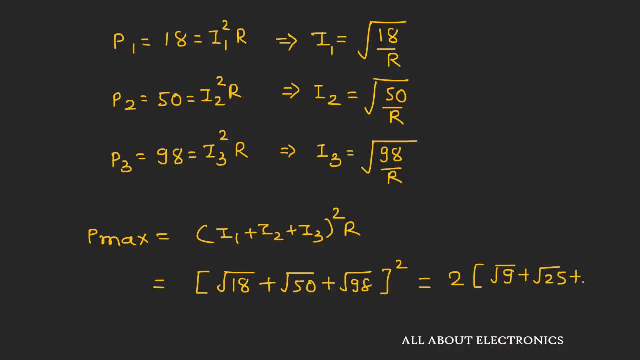 root 9 plus under root 25, plus under root 49.. So we will get the maximum possible power that is 450 watt. So we will get the maximum possible power as 450 watt. So, similarly, let's find out the minimum possible power. So the minimum possible power. 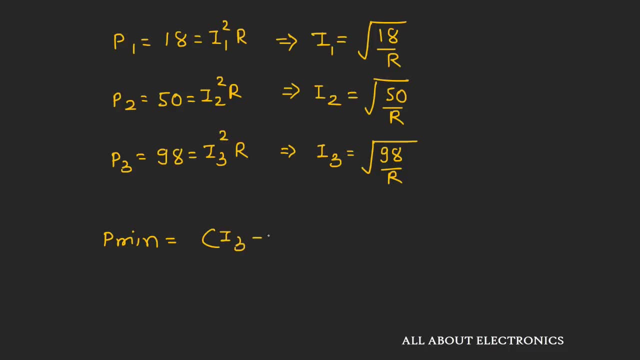 P minimum can be given as I3 minus I2 minus I1 whole square into R. And if we further simplify it then we can write it as a root 98 minus root 50 minus root 18 whole square. And if we further simplify it then we can write it as a 2 into under root 95 plus under. 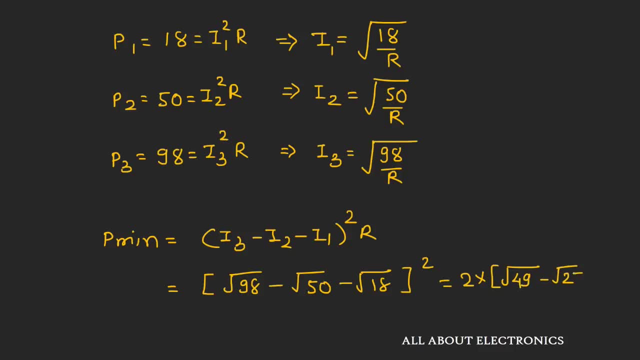 root 49 minus under root 25, minus under root 9 whole square And further. if we simplify it, then we will get 2 into 7 minus 5 minus 3 whole square, So the value of minimum possible power will come out as 2 watt. 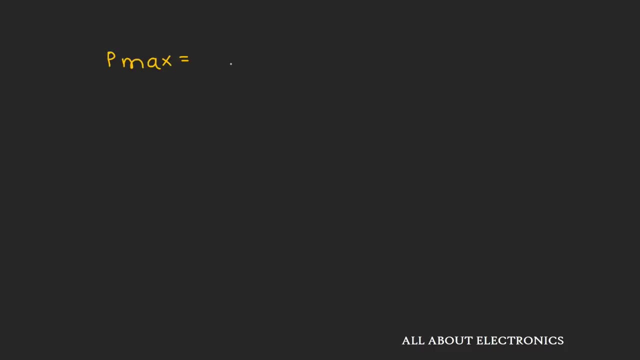 So in this way we found out the maximum possible value as 450 watt and minimum possible power as a 2 watt. So here the point is that for the power calculation we cannot directly use this superposition theorem. So for the power calculation first of all, either we have to find the total current. 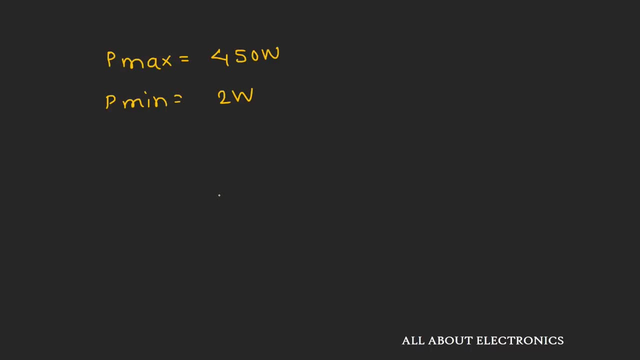 IT or a voltage across that particular element And from that we can find the total power that is dissipated across that particular element. So now let's see the third example. So in this example we have to find the power that is dissipated across this 5 ohm. 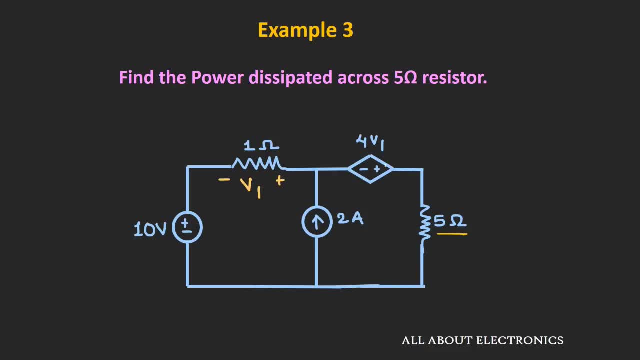 Now, in this circuit, as you can see, we have one dependent source. So, as we have discussed earlier, if the circuit contains a dependent source, then for the superposition analysis we will consider this voltage source ON during the analysis. 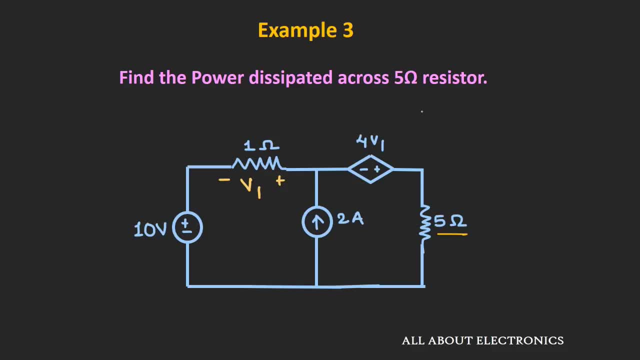 Now here to find the power that is dissipated across this 5 ohm resistor. what we will do? We will find the total current I that is flowing through this 5 ohm resistor. So to find this total current I we will use the superposition theorem, And for that 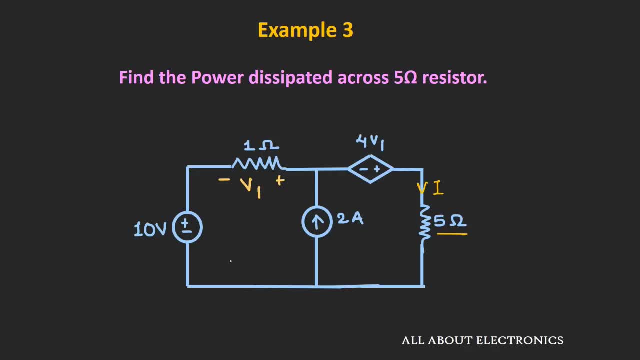 we will consider only one particular source at a time. So first of all we will consider: this 10V voltage source is acting alone. So in the circuit, if only this 10V voltage source is acting alone, then we can replace. 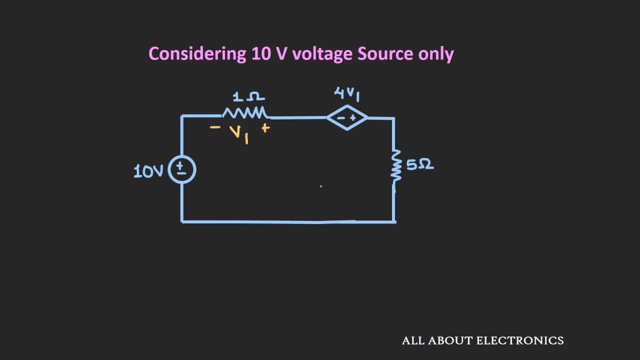 this 2A current source by an open circuit, And the equivalent circuit will look like this: So now let's assume that the current that is flowing through this 5 ohm resistor is I1.. And let's assume that the voltage across this 1 ohm resistor is V1', and hence the voltage 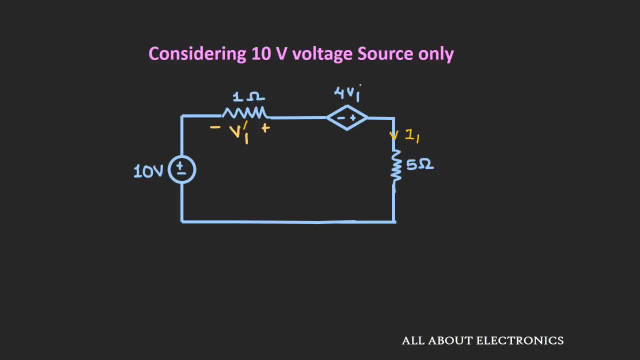 is V1', So the voltage of this dependent source will be V1'. So we can apply a KVL in this loop. So now if we apply a KVL, then we can write it as 10 plus V1' plus 4V1' minus 5I1.. 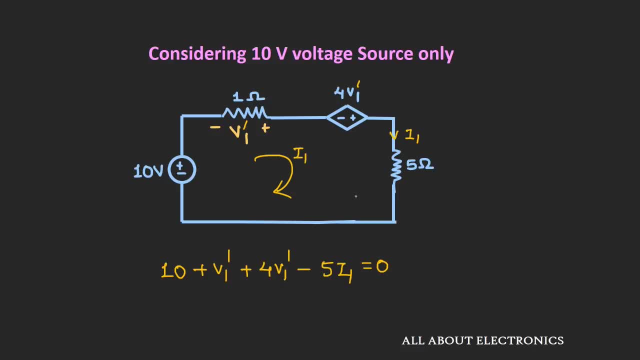 That is equal to 0.. Now, closely, if you look here, this V1' is nothing but minus I1.. That is a drop across this 1 ohm resistor. So we can replace this V1' by a minus I1. 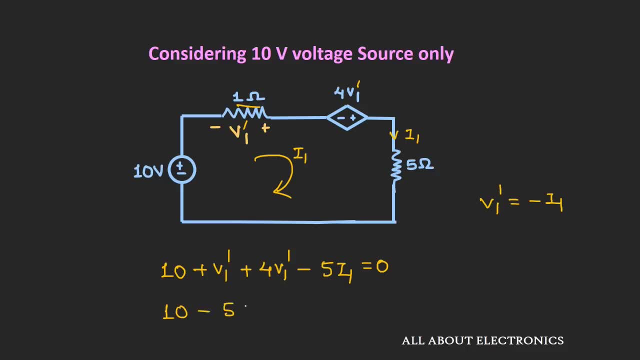 So we will get 10 minus 5I1. minus 5I1, that is equal to 0.. Or we can write I1 as 1A, So in this way we found the current I1 that is flowing through this 5 ohm resistor when. 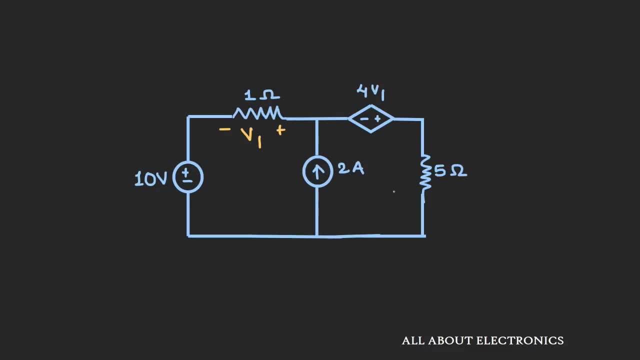 this 10V voltage source is acting alone. Now let's find out the current that is flowing through this 5 ohm resistor when this 2A current source is acting alone. Let us assume that the current that is flowing through this 5 ohm resistor is I2.. 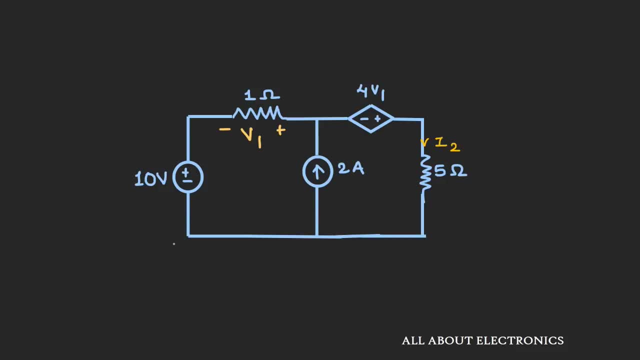 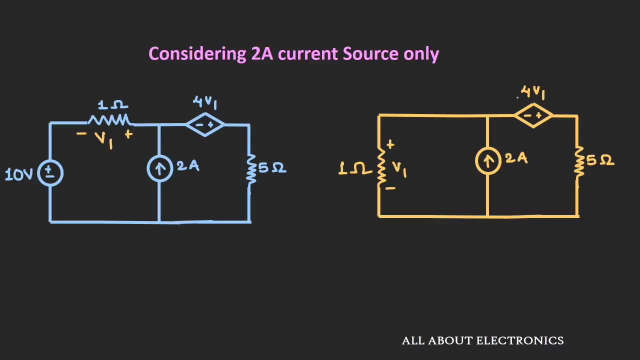 And in that case we can replace this 10V voltage source by a short circuit. In that case, the equivalent circuit will look like this, And let us assume that the voltage across this 1 ohm resistor is nothing but V1'. 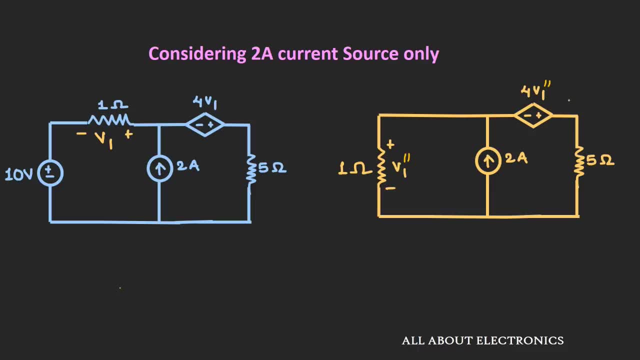 And the voltage of this dependent source is 4V1'. So if you see this circuit, we have total two nodes. This is the first node and this is the second node. Let us assume that the voltage at this node is V1''. 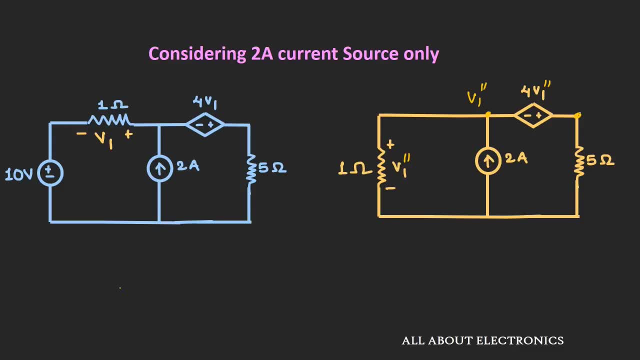 That is the voltage across this 1 ohm resistor. And let us assume that at this end the voltage is nothing but V2.. And the current that is flowing through this 5 ohm resistor is nothing but I2.. So if you see, here between these two nodes we have a super node. 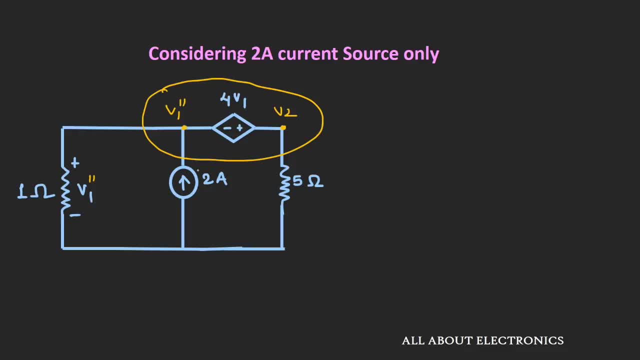 So we will consider these two nodes as a super node And let's apply a KCL for this super node. By applying KCL, we can write V1'-2A plus V2'5, that is equal to 0. Now, here I2 is nothing but V2'5, where I2 is the current. that is flowing through this. 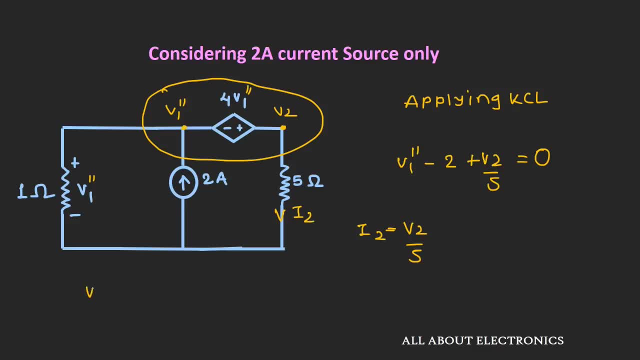 5 ohm resistor. Now for this super node. we can write V2-V1' that is equal to 4V1'. Or we can write: V2 is equal to 5V1'. Now, if we put this value in this equation, then we will get: I2 is equal to V1'. 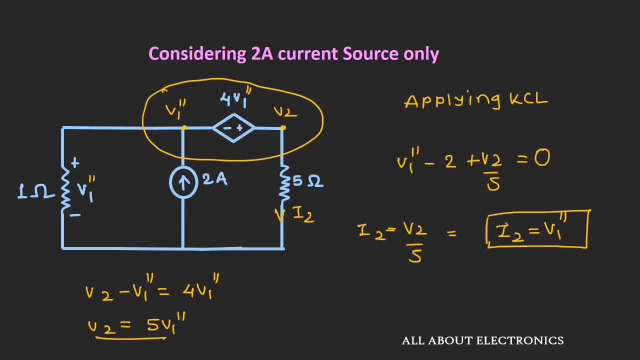 And if we put this value in this first equation, then we will get I2-2 plus I2. that is equal to 0.. Or we can say that I2-2 plus V2' is equal to 0.. say that I2 is equal to 1 A. So in this way we have found the value of current, that is. 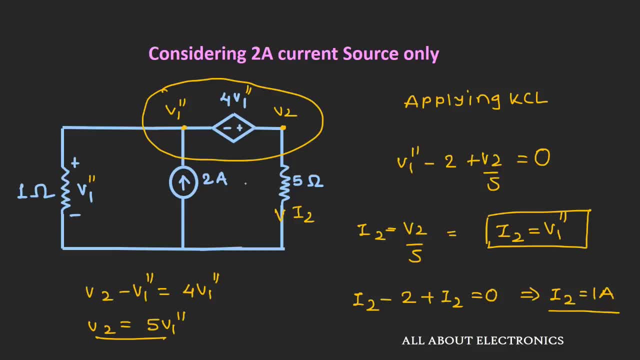 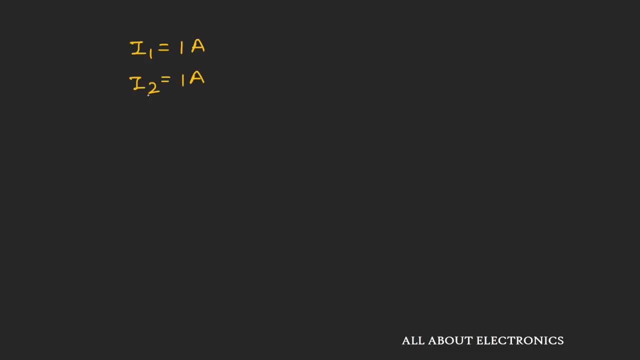 flowing through this 5 ohm resistor when this 2 A current source is acting alone. So in this way we found that value of I1 as 1 A and value of I2 as also 1 A, So the total current I that is flowing through this 5 ohm resistor is nothing but the algebraic. 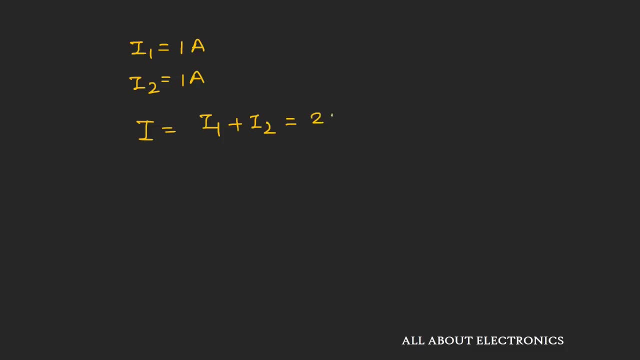 sum of these two currents, that is 2 A. So in this way the total current I that is flowing through this 5 ohm resistor is nothing but 2 A. So now the power that is dissipated across this 5 ohm resistor is nothing but I2 into. 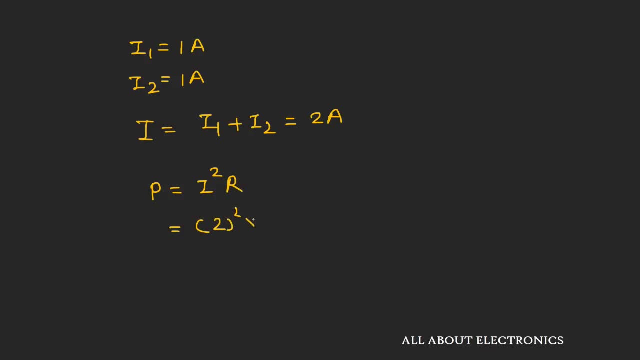 R, That is 2 square into 5. That will come out as 20 V. So in this way we can find the power that is dissipated across this 5 ohm resistor. So in this way, using this superposition theorem, we can find the power that is dissipated. 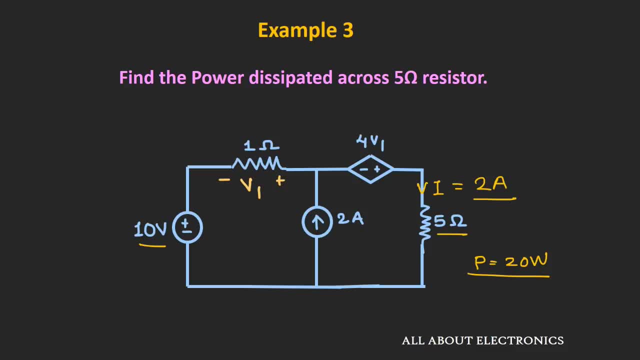 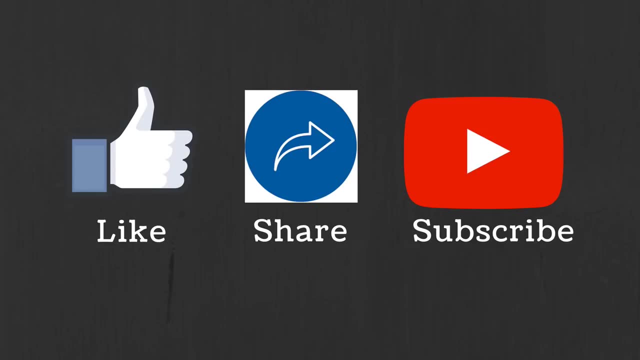 across this 5 ohm resistor. So I hope in this video you understood what is superposition theorem in the electrical circuits And, using this superposition theorem, how we can solve the circuit problems. So if you have any question or suggestion, 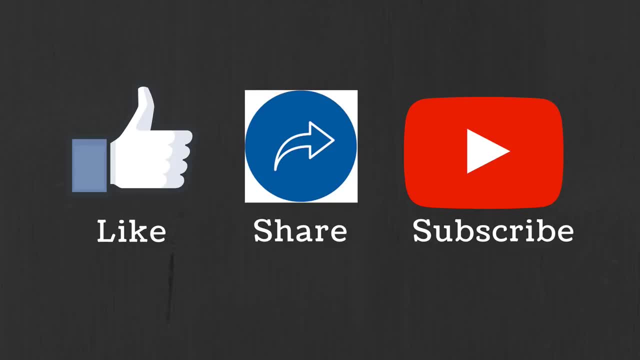 please let me know in the comment section below If you like this video. hit the like button and subscribe to the channel for more such videos.